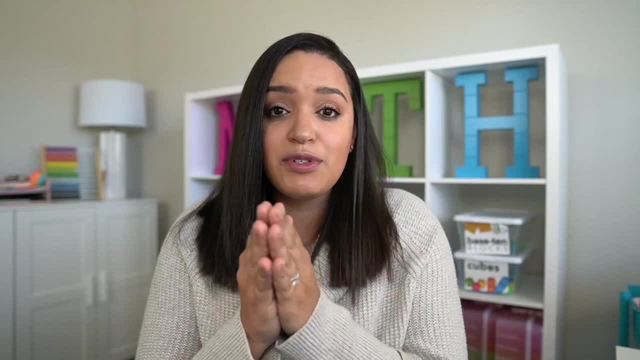 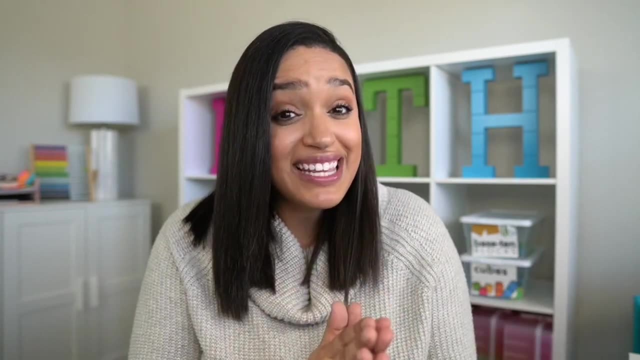 working on multiplying a whole number times a fraction, that three times two thirds. it's pretty easy for students to understand and visualize and model. Now, one thing that's really important- and you'll see this throughout this video- is that we provide context to the numbers. So let's think: 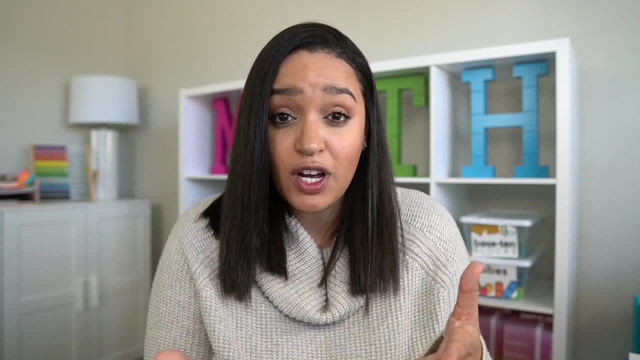 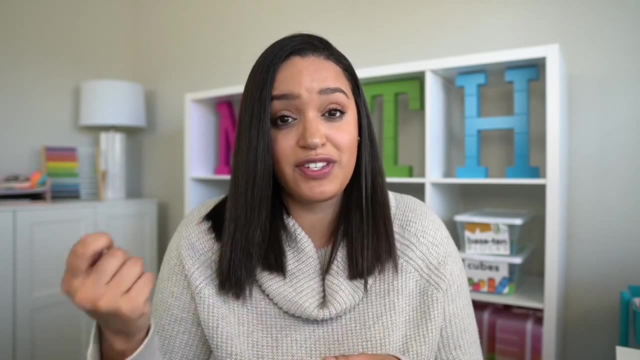 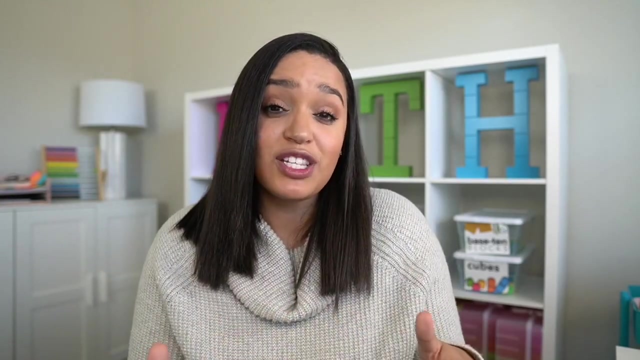 of three times two thirds, as three scoops of dog food and each scoop is two thirds of a cup. so we two thirds of a cup and another two thirds of a cup and another two thirds of a cup, And that is three groups of two thirds. So that is multiple groups. Let's take a look at what this looks like. 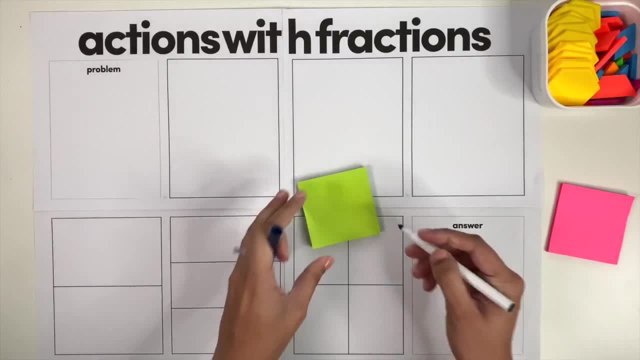 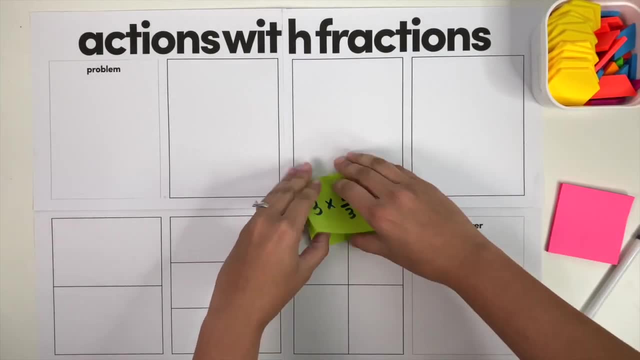 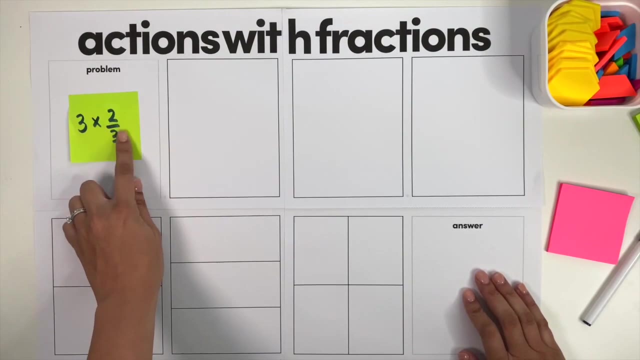 to model it with pattern blocks on our math mat. Okay, So we are going to model three times two thirds, which in this situation, we know is three groups of two thirds because we are working with multiple groups or equal groups, And so we've got three groups of two thirds. Let's go ahead and 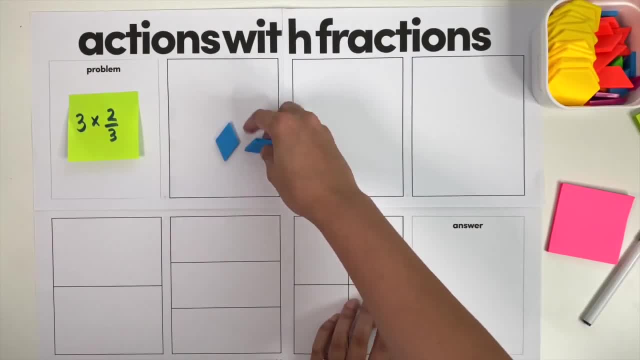 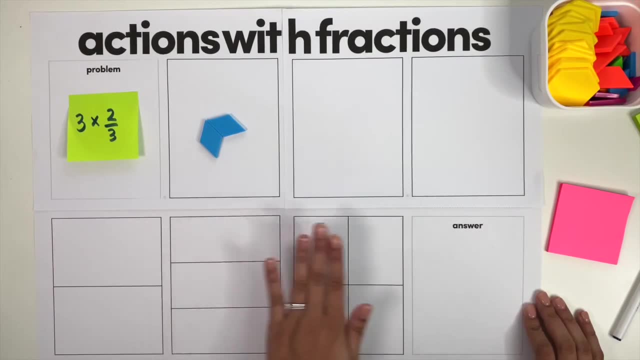 model one group of two thirds And so this would be one group. And if you look at our math mat, here we've got three whole groups up, here We've got halves, thirds and fourths, And so we'll be using 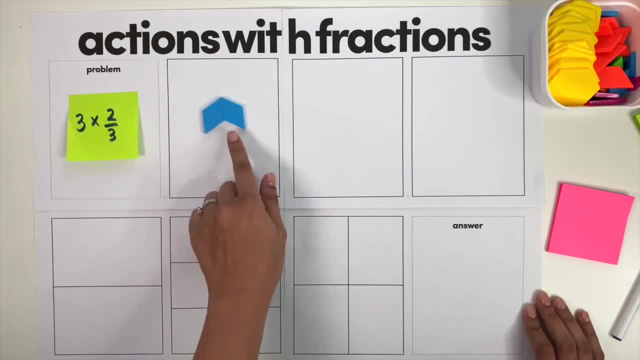 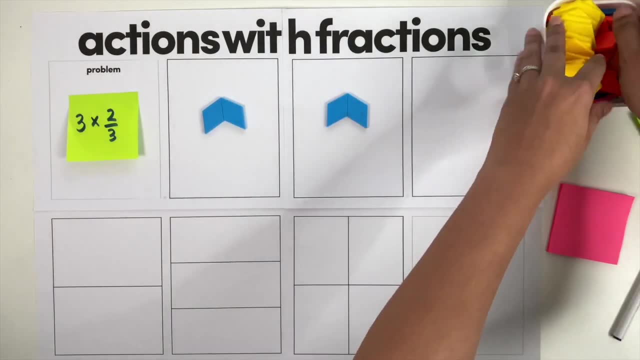 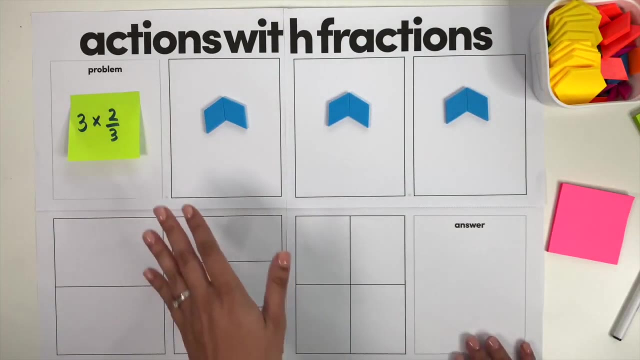 that throughout this activity. So here we've got one group of two thirds, We've got another group of two thirds, And then we have another group of two thirds, And so to figure out what the total number of two thirds is, we're going to model one group of two thirds, And so we're going. 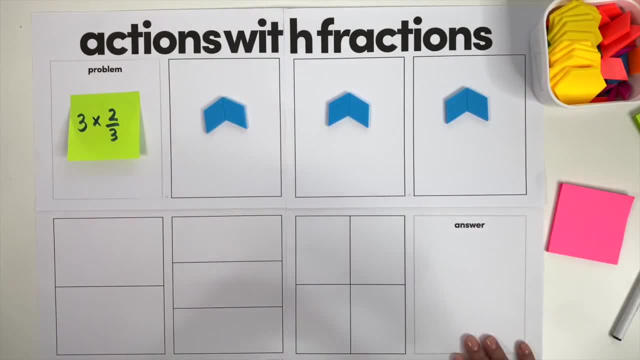 to use that total value of three groups of two thirds. Let's see what the total value of three groups of two thirds are. We need to go ahead and combine them for our answer. So I could say that it's six thirds. Put our answer sticky note here. I could say that it is six thirds because we know. 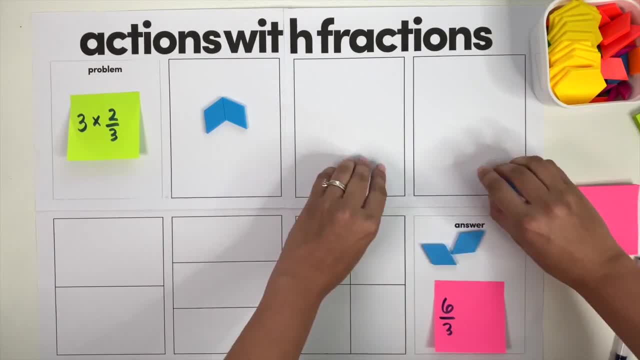 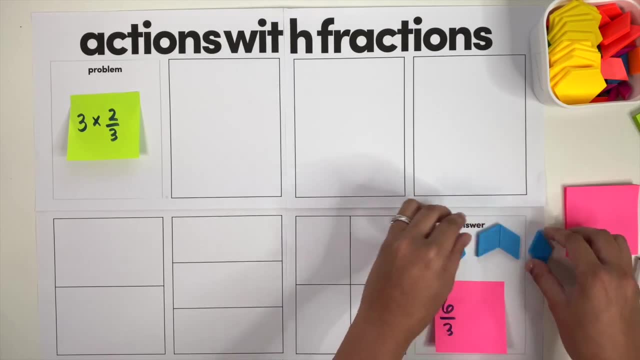 that all together we've got six thirds here. One, two, three, four, five, six. Or if I were to do some regrouping here, I could see that six thirds is also two wholes. So our answer is six and six thirds or two. Now that students have grasped what it looks like to 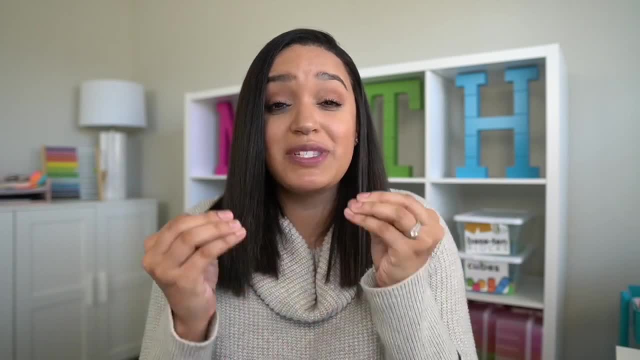 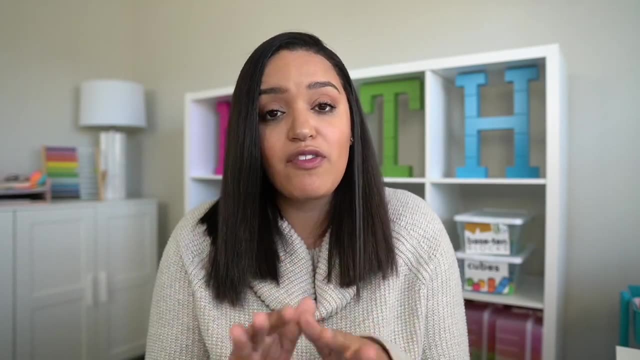 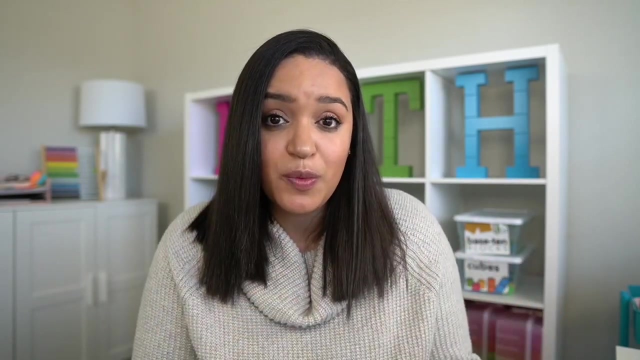 solve multiplication problems with fractions in a multiple group situation. that is typically where most fourth grade standards stop. But there is another type of multiplication situation that we can fall into with multiplying a whole number by a fraction, and this is partial groups. So instead, 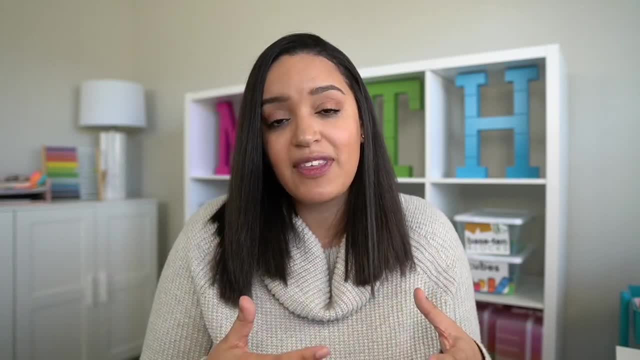 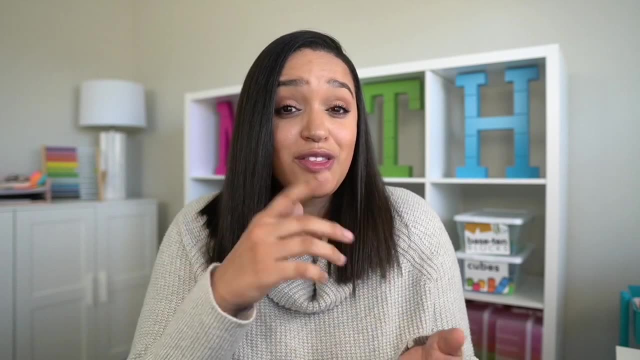 of three groups of two thirds. we're thinking about this in a two thirds of three situation. This is why context is key, because on paper, three times two thirds and two thirds times three, they have the same product. so how are they different? But let's add a little context and 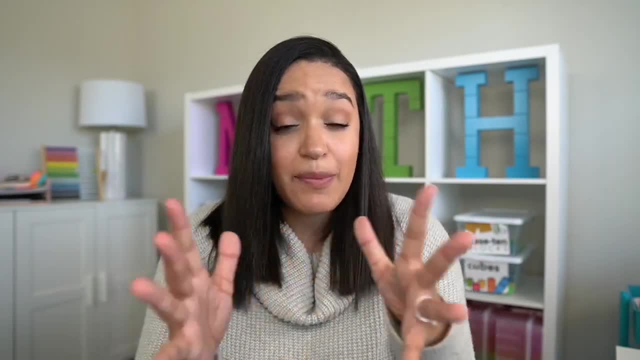 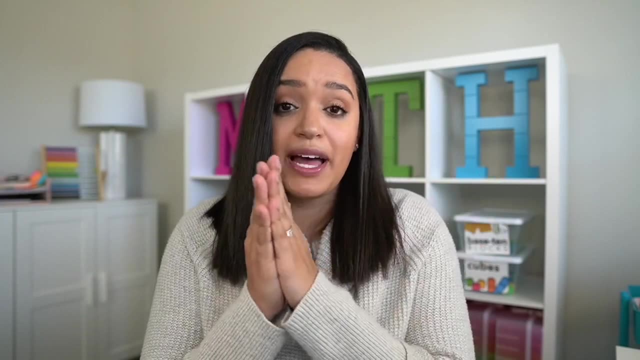 you'll see very clearly how these two things are different. So when we're talking about this partial groups type of thinking, let's start with part of a group, So a fraction by a whole number. So let's use the same context We've got. 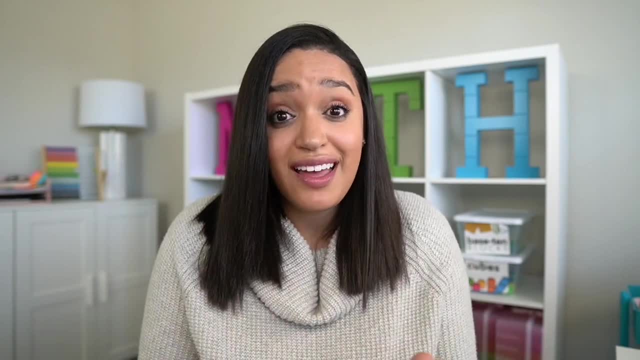 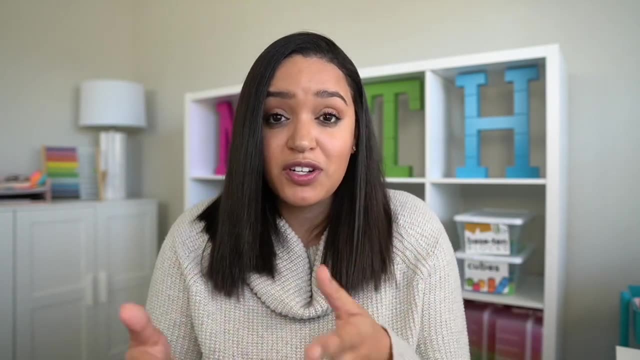 three cups of dog food, so two thirds of the three scoops of dog food were spilled. Now, the reason this isn't multiple groups and the reason we wouldn't model it as two thirds and two thirds and two thirds is because let's think about this in this situation, If we were to view 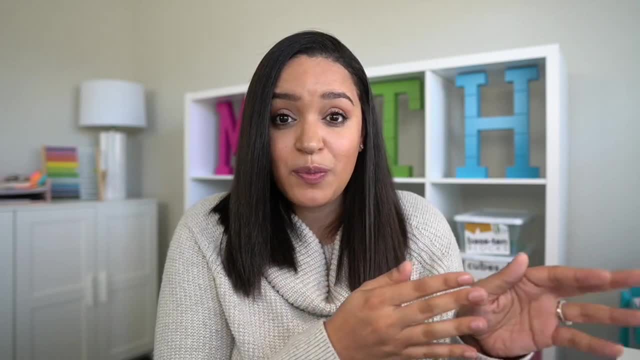 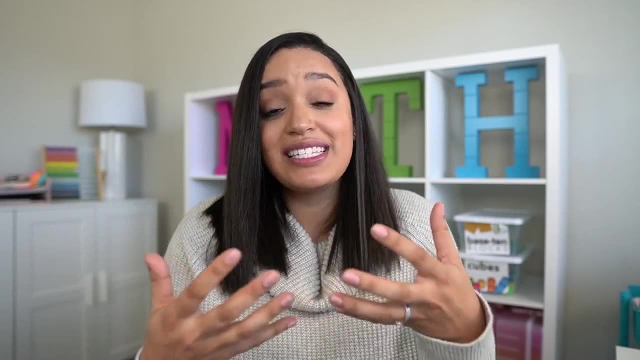 it as multiple groups. that would mean that two thirds of this scoop was spilled and two thirds of this scoop was spilled and two thirds of this group was spilled, And that's not the case here. What it's saying is: we're taking part of this group of scoops and two thirds. 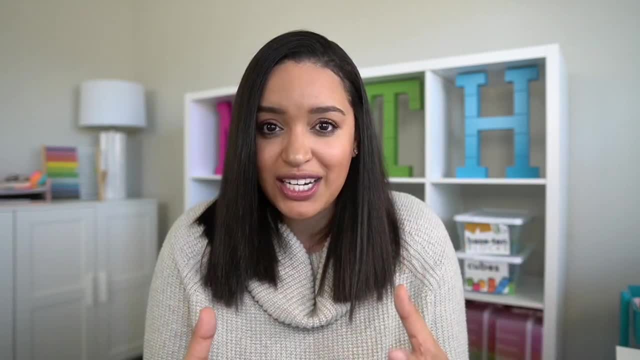 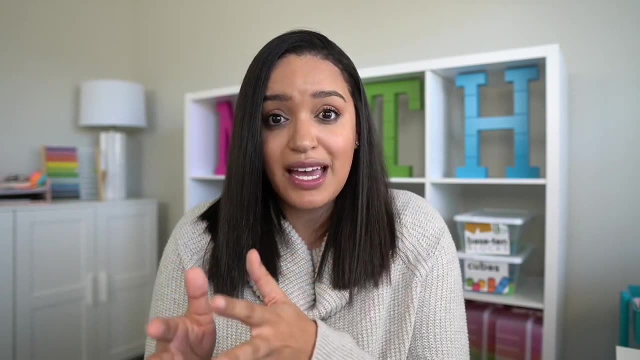 two thirds of them were spilled. So it's a different type of action here and it's a different type of thinking, And that's why in most states with most standards, this is a fifth grade concept. A lot of times, teachers who are expected to teach multiplying a whole number by a fraction. 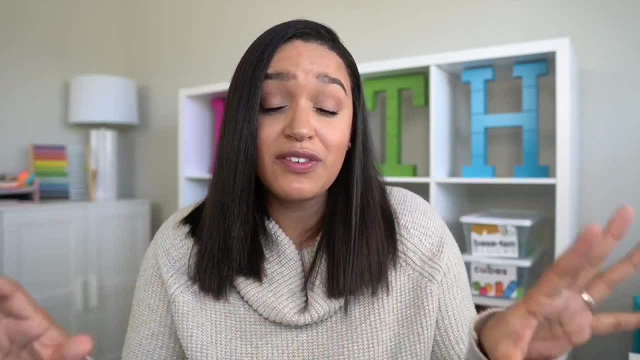 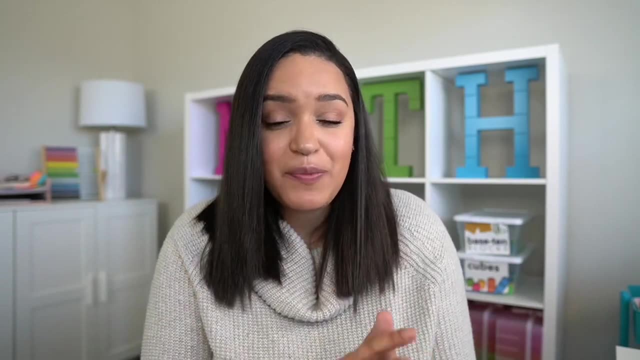 will kind of pull problems and not realize that these are two different types of thinking, one of which students may not be ready for. So in just a sec I'm going to show you how to model this with our pattern blocks and our math map. But before we do that, I want us to focus on 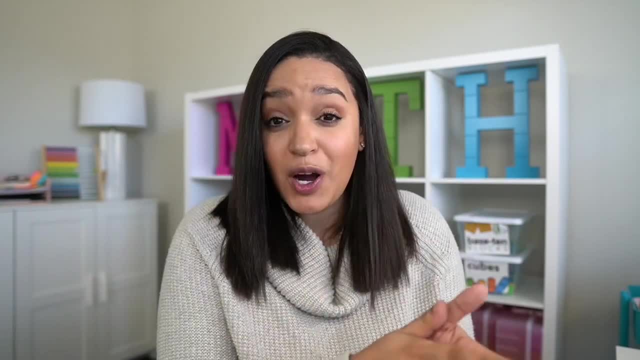 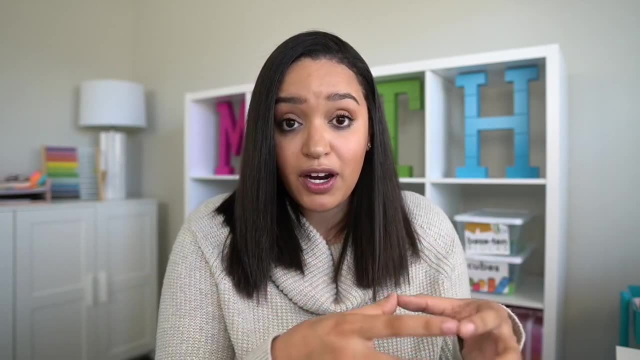 another type of partial groups type thinking and that is part of a part, And so that just means still kind of the same thing We're finding instead of part of a group, we are finding part of another part. So instead of two thirds of three, maybe it's two thirds of one half. 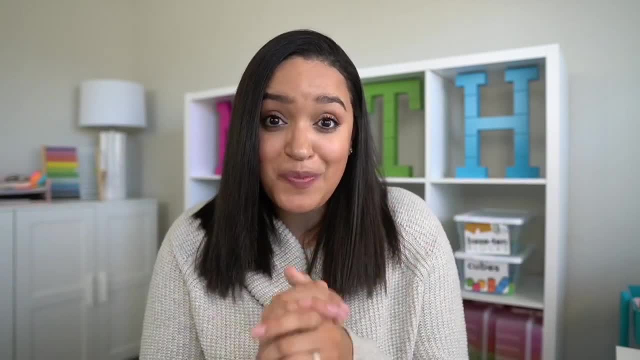 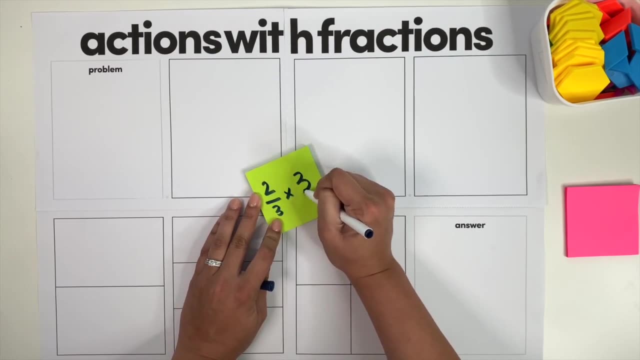 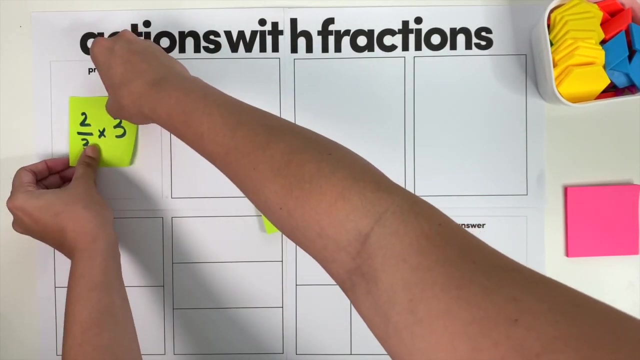 So we're going to look at both of these problems with our math map and our pattern blocks now, All right. So let's take a look at two thirds of three, or two thirds times three. In this situation, two thirds of the three cups were spilled, So let's go ahead and model three cups. 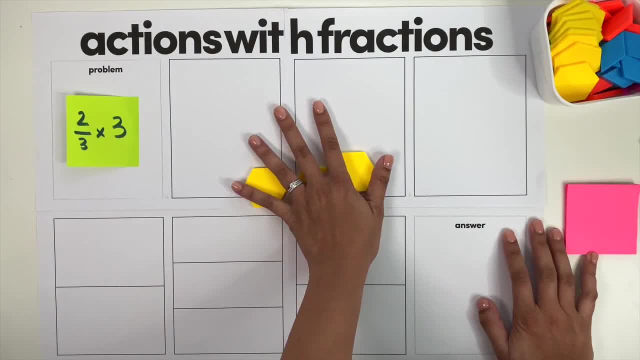 So three cups would be three whole cups And we want to split this group right here into thirds. So let's go down here and take a look at our thirds. And we know, if we were to split this into thirds, one whole would be in each third. Now we want to look at two thirds of this group. 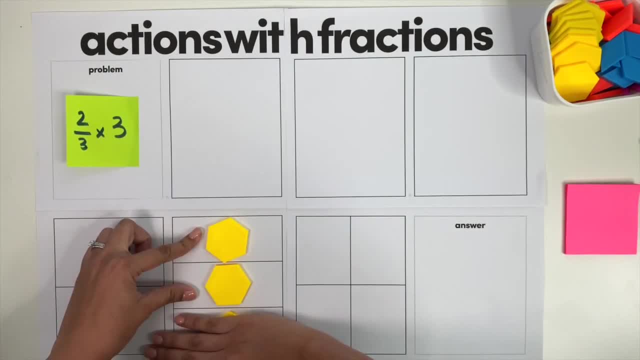 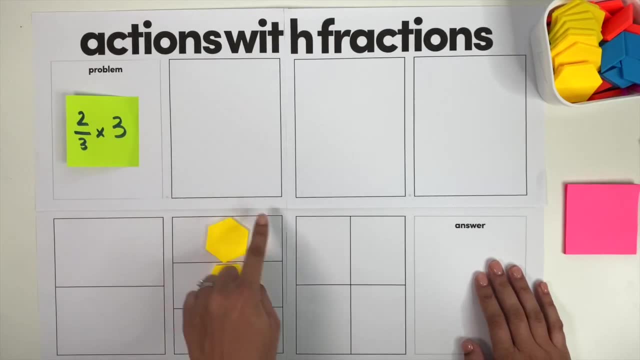 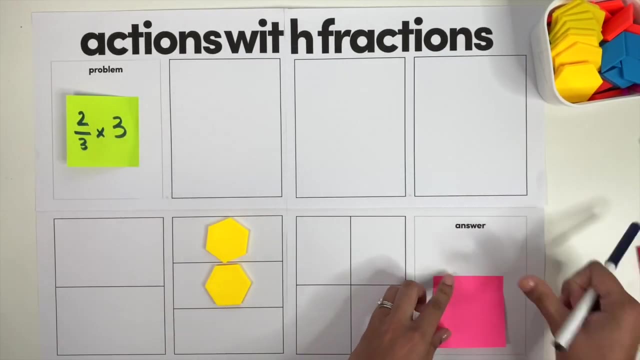 And so we will look at just these two thirds. So we need this final third. So we can see here that two thirds, one third of three, would be one, two thirds of three would be two. We can see that two thirds of three is actually two wholes. 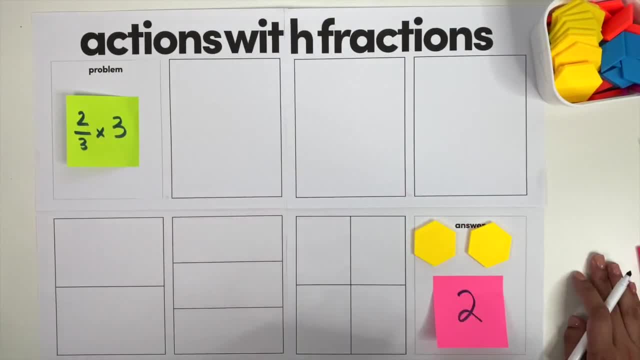 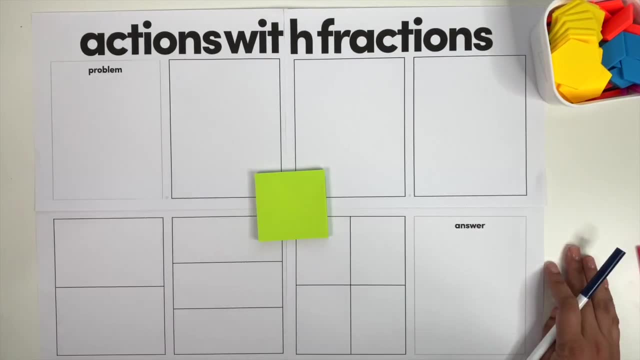 So it said that two thirds of the three cups had been spilled. How many cups had been spilled? Two whole cups. Now. the second problem I mentioned was part of a part. So instead of finding part of a group- so two thirds of three- now we're looking at part of a part, And so let's take a look at how. 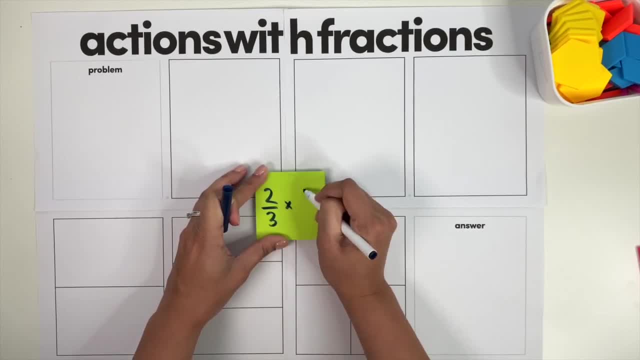 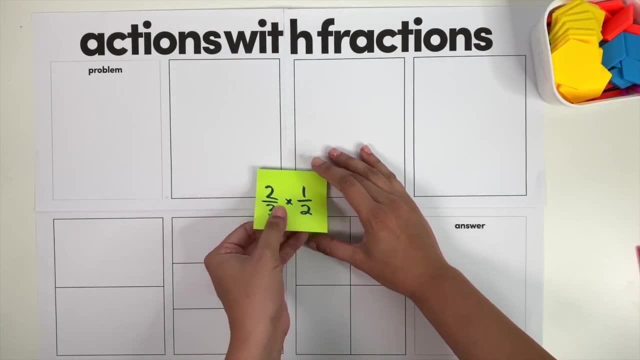 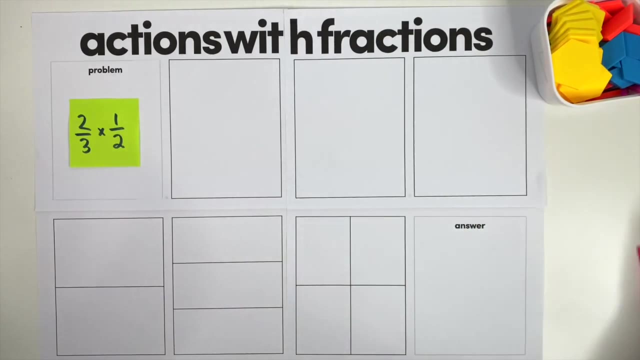 we would model two thirds times one half, So two thirds of one half. So if we're adding a little bit of context to this situation, we could say that the dog ate two thirds of a bag of dog food and the bag of dog food was a half a pound, So he ate two thirds of that half pound. 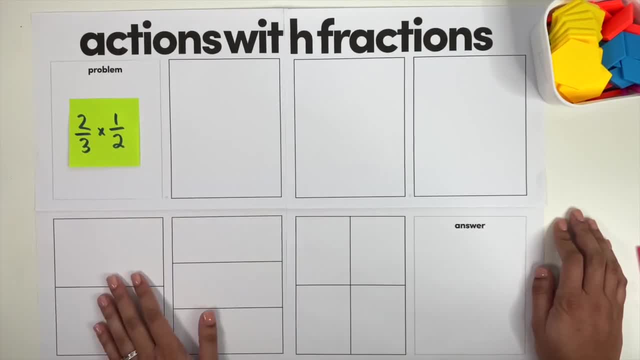 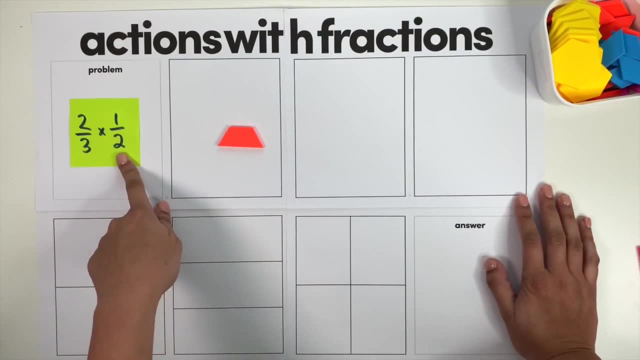 How much did the dog eat? Let's start by modeling one half. So we've got one half here and we want to find two thirds of this. So just like we had to split the three wholes that one group, we had to split three wholes into. 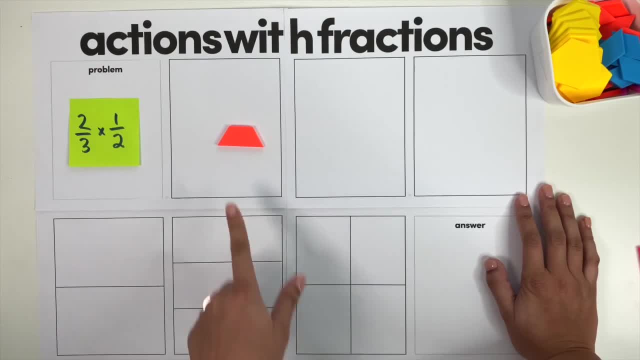 thirds. Well, now we need to split this half into thirds, And so we can't do it the way it is, So we'll have to do a little bit of replacing, And so I know that I can turn this into sixths, because 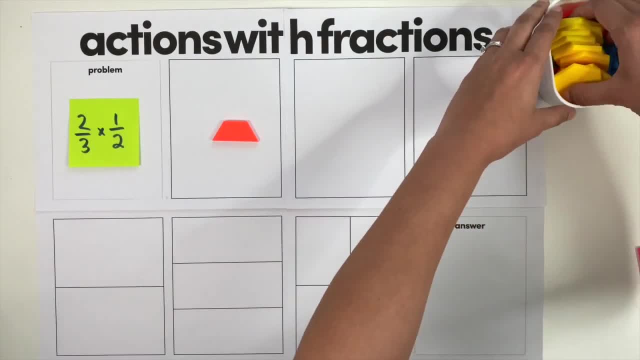 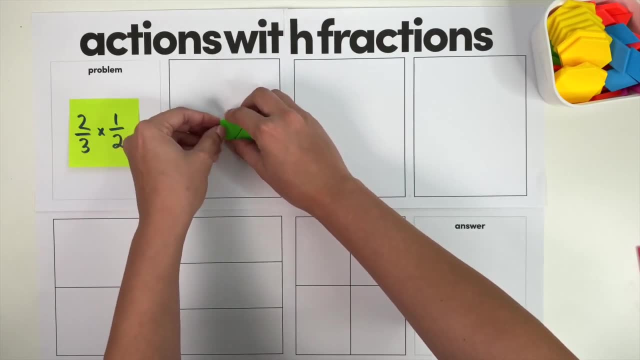 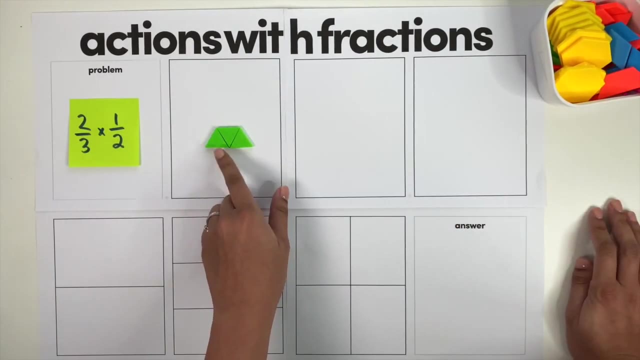 one half is equivalent to three sixths, So let's go ahead and do that. Okay, So I'm going to exchange. you can see, I'm going to exchange this one half for three sixths. So this is still finding two thirds of a half. This is still a half here, but now we can split it into thirds. 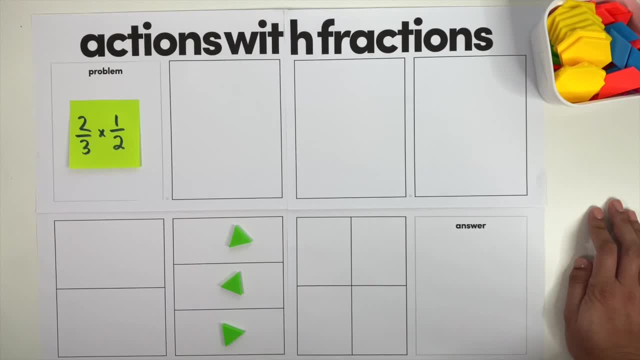 So let's go ahead and split it into thirds And, just like our last problem, we want two thirds of this. So one third of one half would be one sixth, Two thirds of one half would be two sixths and three thirds, or a whole group of one half would be three sixths, which is one half, So that 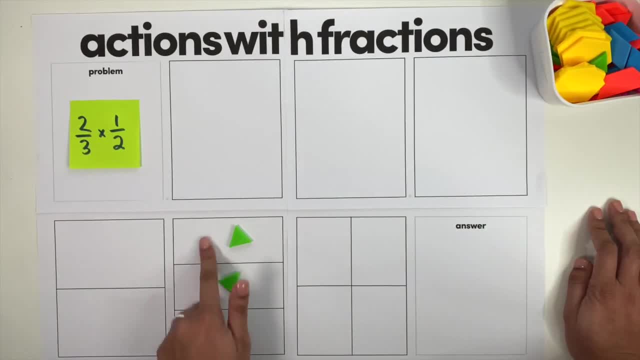 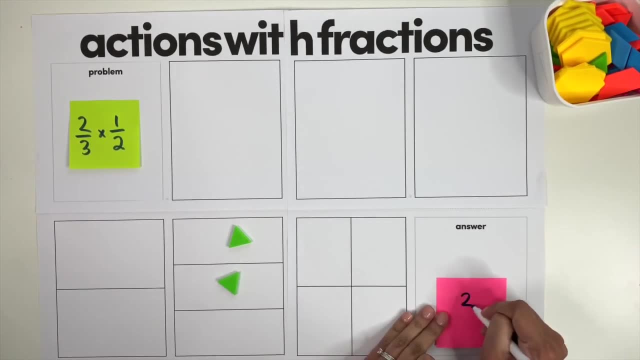 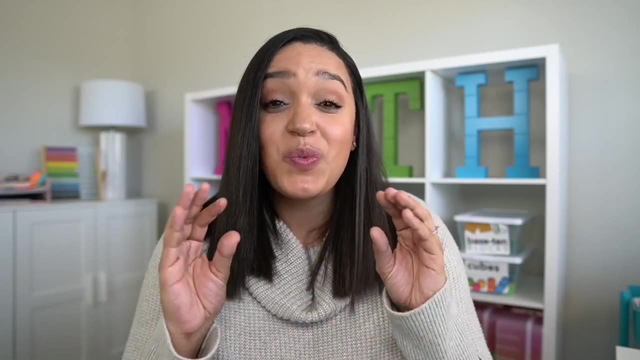 makes sense. So let's take this away, because we only want two thirds. And so here I can see that two thirds of one half is two sixths, And so here we have found part of a part. All right, there's one last step. 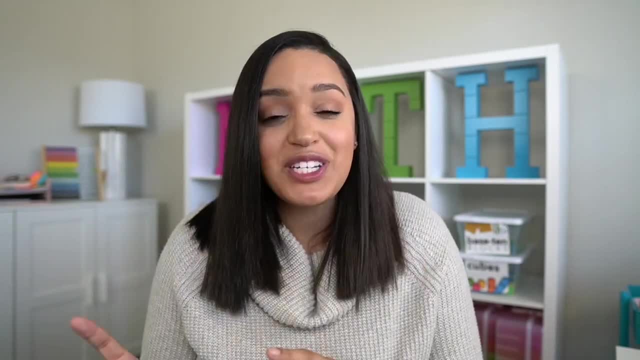 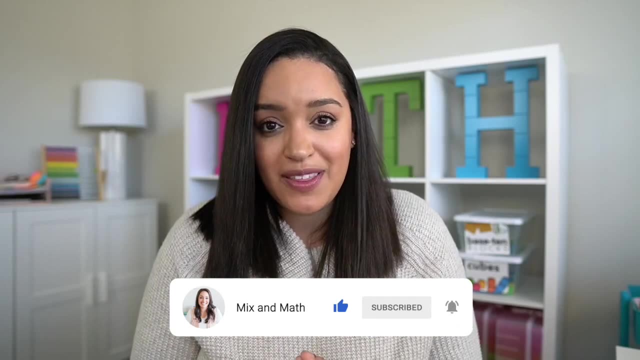 in the progression for multiplying fractions. But before we jump into that, I want you to take a second to like this video and subscribe to my channel. if you have learned something new up to this point. I'd love to know if this is helpful, because then I know that I can make more videos like this in the 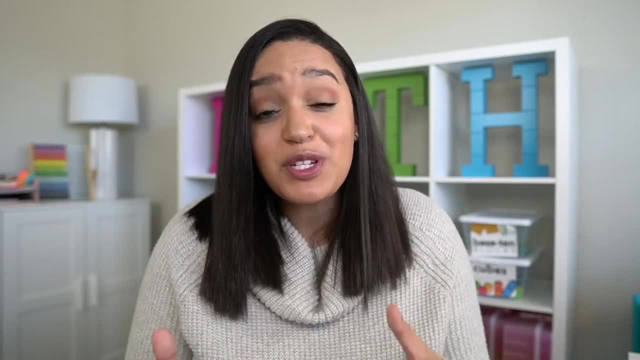 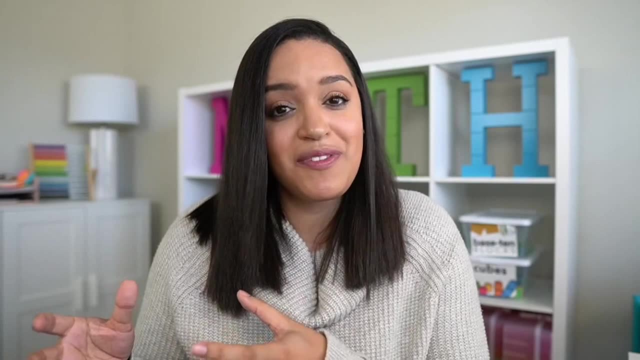 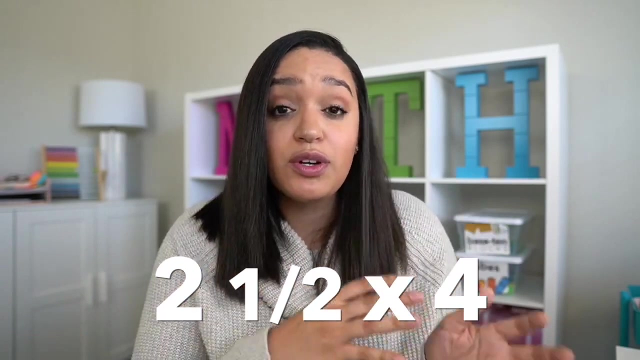 future. Okay, so the very last step in the progression for multiplying fractions is really just mix and matching the multiple groups type of thinking and the partial groups type of thinking. So what this looks like is, let's say, two and a half times four. Well, two and a half times four is two groups of. 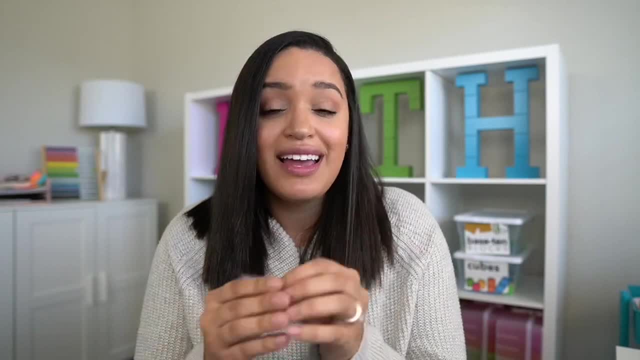 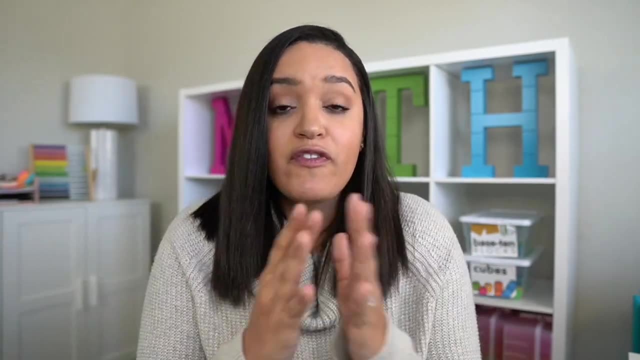 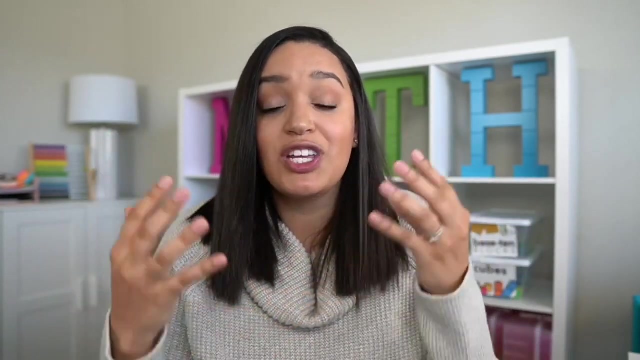 four and half of four. So two groups of four, multiple groups, half of four, that partial groups type thinking. So you could do that. you could do four and a half times one. fourth, that is multiple groups and part of a group. So you're really just mixing and matching these two types of thinking to really solve any fraction. 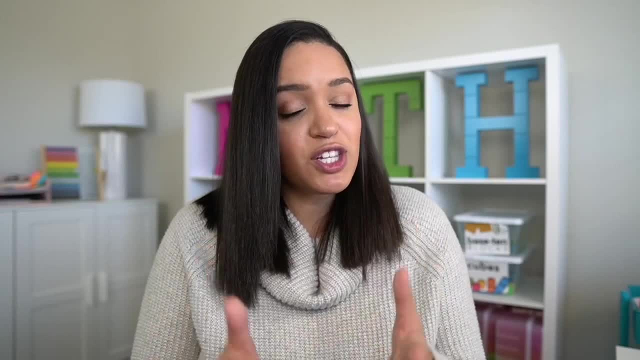 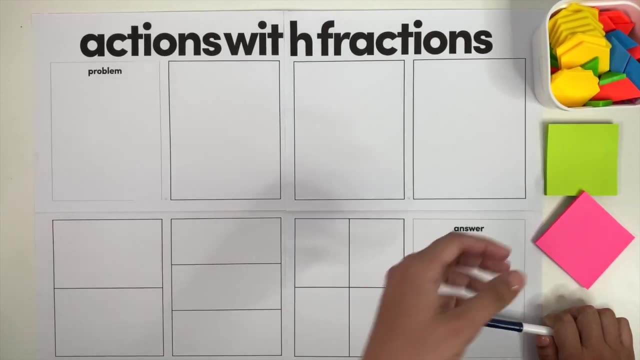 multiplication problem that students are given. So one last time, let's look at our math mat and our pattern blocks to see how we would model these problems. So our very last step in this progression is combining both types of thinking. So let's take a look at two. 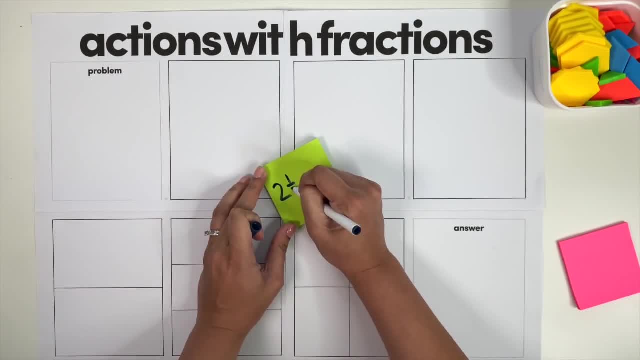 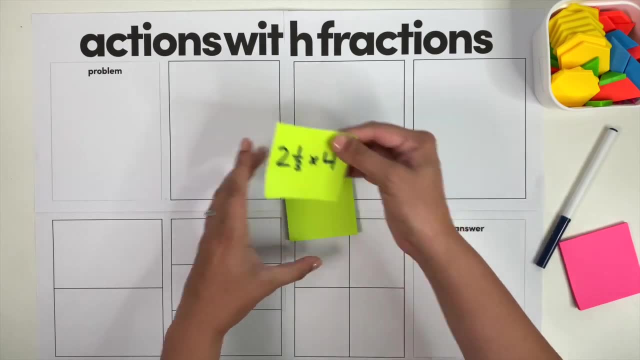 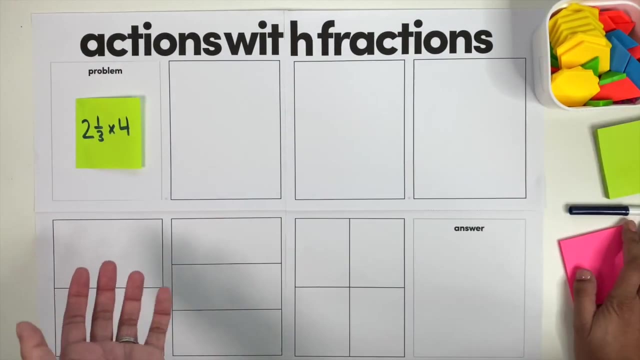 and one third times four. So two and one third times four, This is two and one third groups of four. So in this situation it might be that throughout the week the dog ate two and one third containers of dog food and inside each container 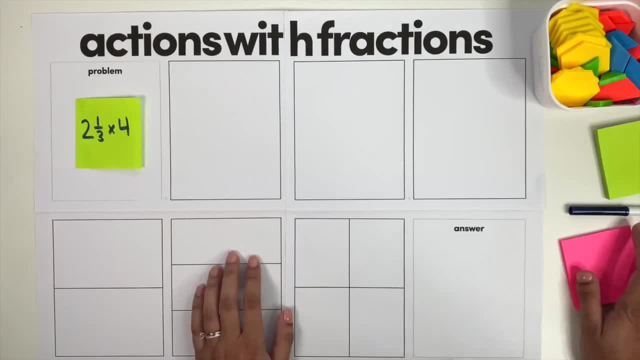 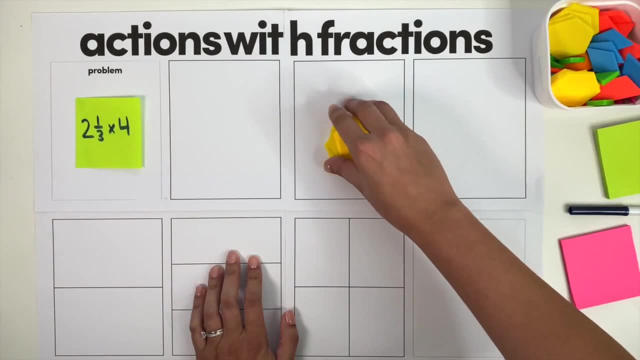 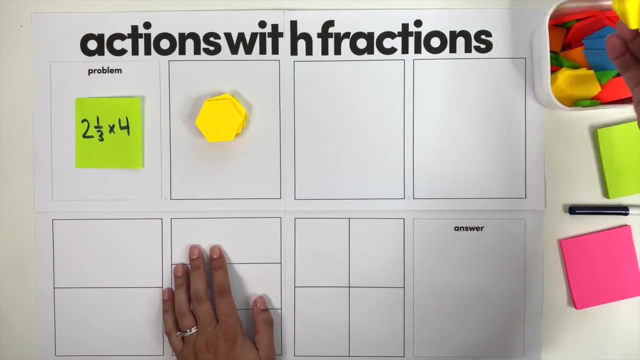 there was four pounds. So we've got two and one third groups of four. So let's go ahead and start by modeling four. Okay, so we've got two and one third groups. So here's one group. We need a second group. So we've got two groups of four. 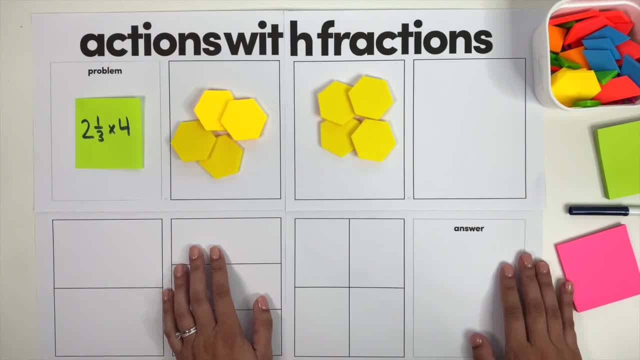 I'll spread them out so that way y'all can see them. So so far we've modeled two groups of four. Now we need one third of a group of four, or one third of four. Well, let's take our four here And we need to split it into thirds. we may have to do some exchanging here. 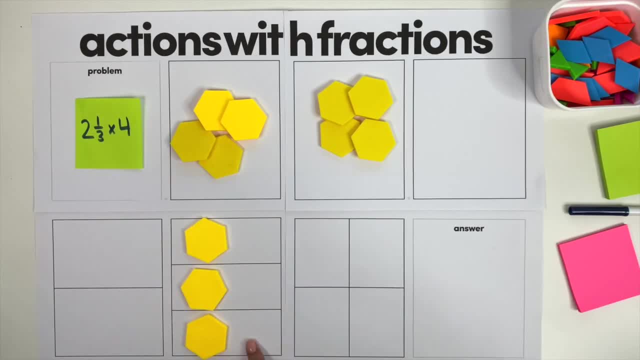 So let's see, I know I can put one hole into each of the thirds, So now I've got to figure out a way to split this hole into thirds here, because we know that we've got to have these in equal groups. So I'm going to exchange it for. 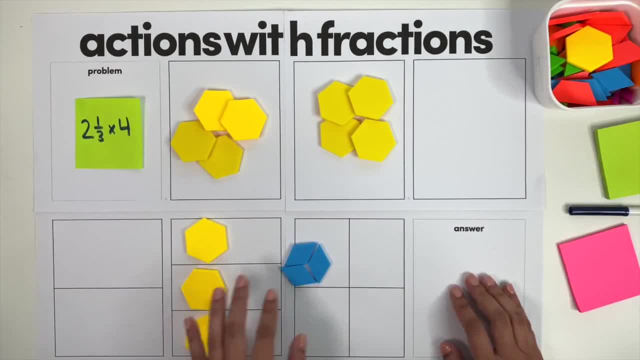 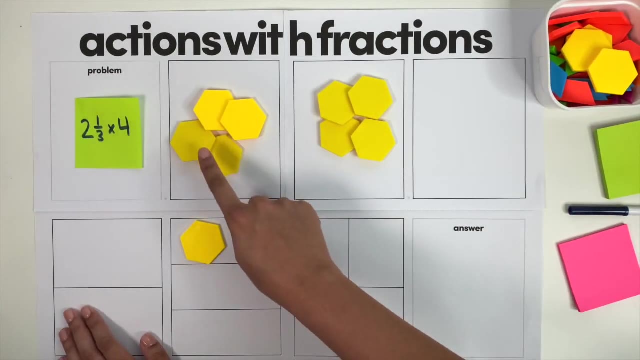 thirds right here. So I've still got four holes here, But now I can put them into thirds, And we want one third of four, So we just need this section right here. So I'm going to go ahead and take away these And now I have modeled two and one third groups of four. 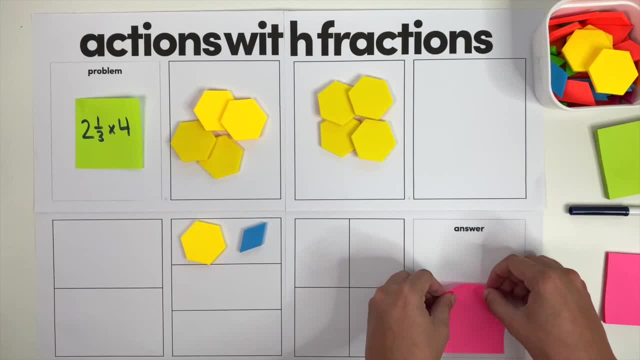 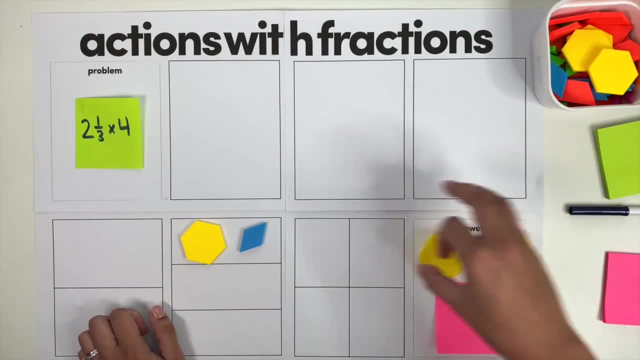 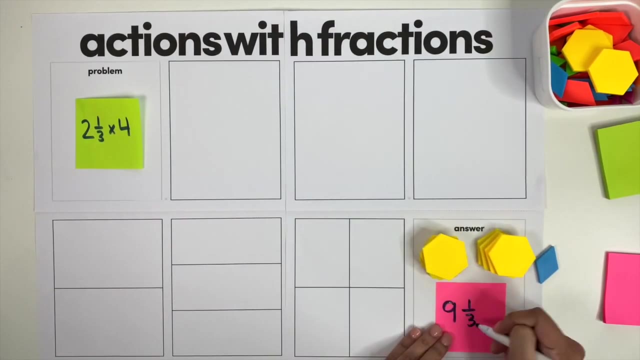 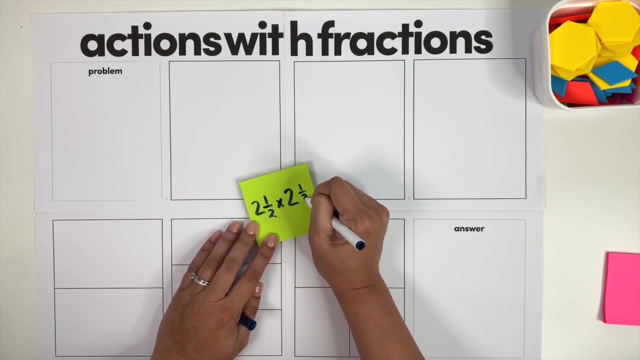 And so our answer. we know we need to combine all of these together. So we've got four, eight, nine and one third. So our answer is nine and one third. So let's look at two and one half times two and one third. So we've got two and a half groups of two and one third. 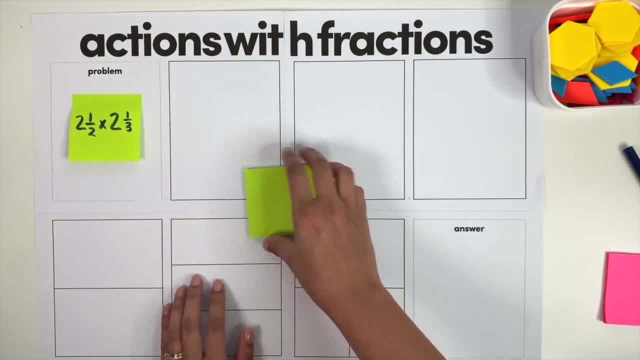 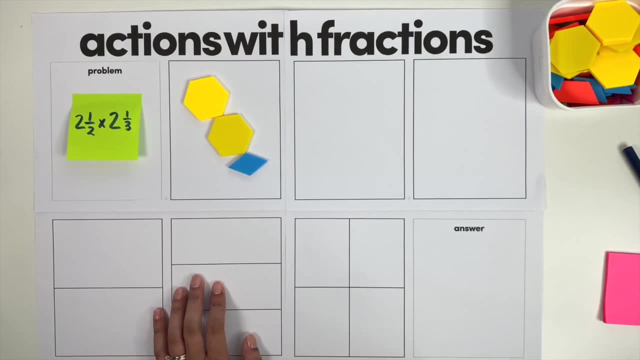 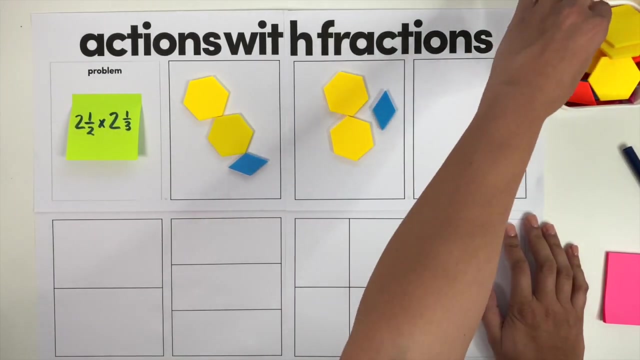 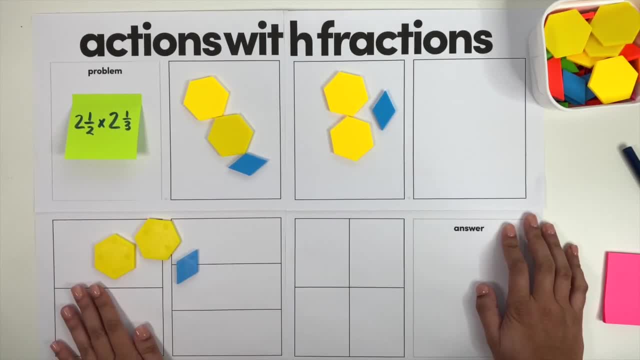 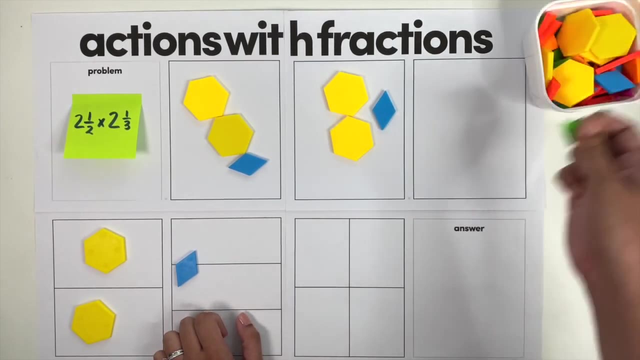 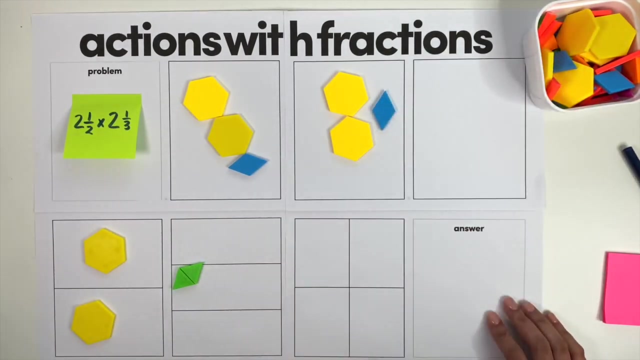 But we need to split this into half. So we are going to go over to our half section here, And so it's pretty easy for me to go ahead and split the two holes into half, because I just put one hole in each of the halves And now I'm going to do a little exchanging here. And so, because I've worked with pattern blocks and I understand them, I know that I can exchange one third with two sixths And that would give me those two pieces. So now I can split this third into two groups. 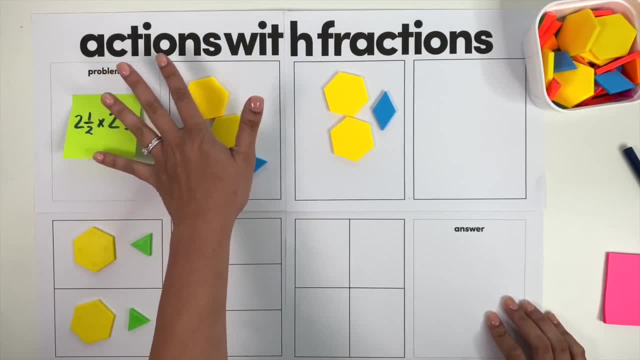 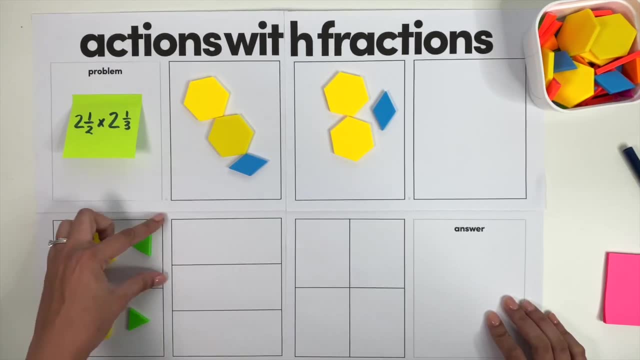 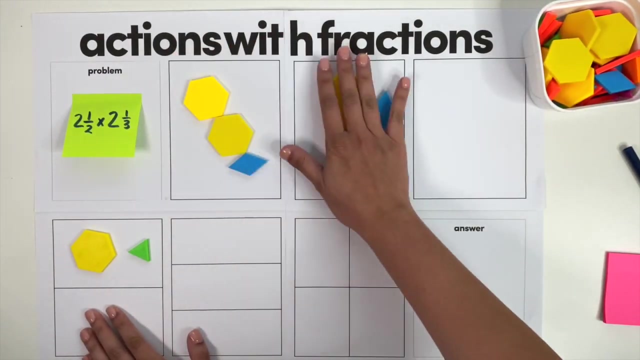 So we're into half Now. so far we've modeled our multiple groups. we've got the two whole groups of two and one third, And so here we just modeled our part of a group by finding half of two and one third. you can see we still have two and one third here. we've just split it in half And we're only looking for one half so I can remove this other half. And now we have successfully modeled two whole groups of two and one third and a half a group of two and one third, And let's combine all of these. So 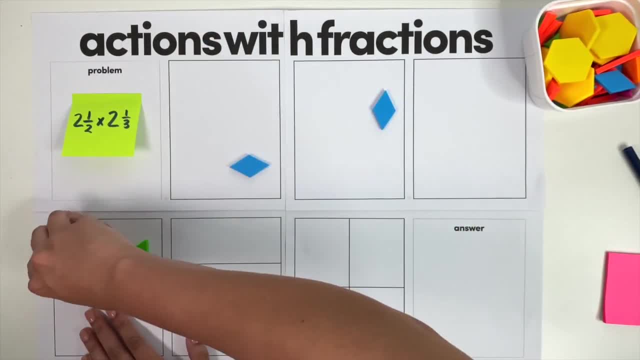 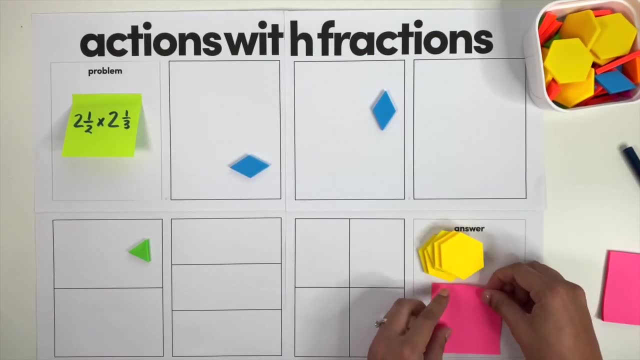 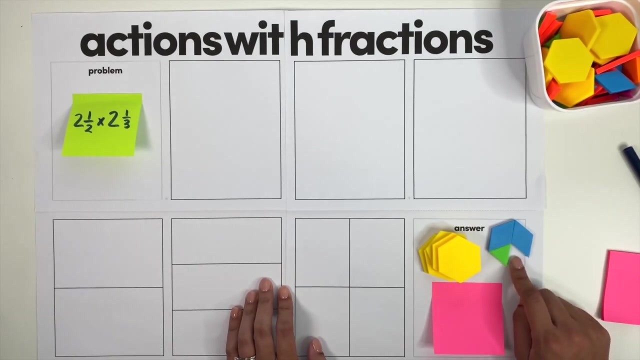 find our answer. So let's take all of our holes here. So I've got 12345.. I've got five holes And I've got these pieces right here. Now there's a couple ways that I could look at this. I could look at this and say, Okay, well, this is one sixth away from a hole, So I know that this is five, six. or I could have exchanged each of these for two sixths and another two sixths. 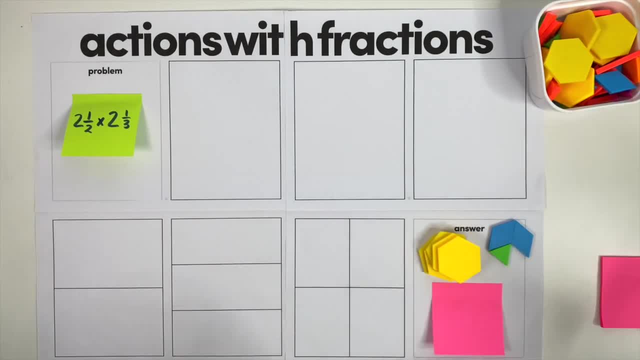 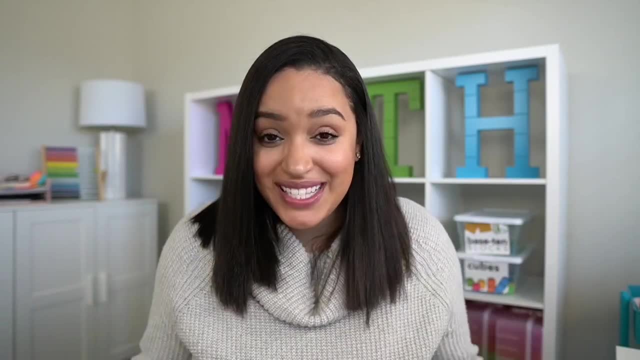 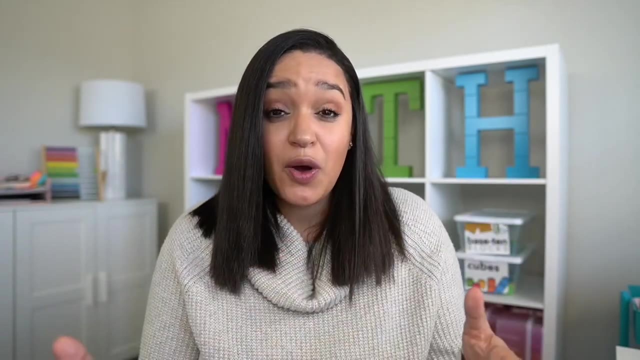 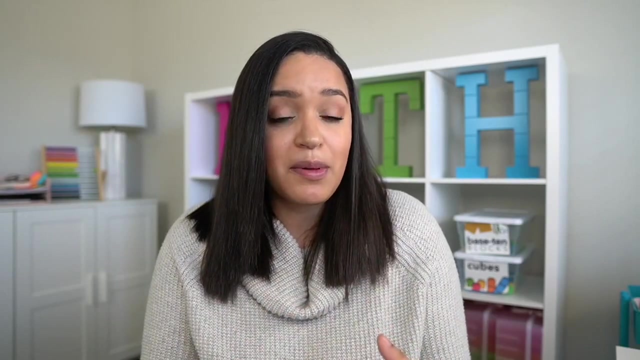 And that would make this last one the fifth six. But either way, I know that my answer here is five and five, six. Okay, that was a lot. But before I tell you how to get this free math mat, I want you to know that, if you loved this video, if you want to know how to make other fraction concepts- hands on- and you want to actually see it in action, with me modeling these problems out, I want you to take a look at Mixing Math 360.. That is, our memberships exclusively for